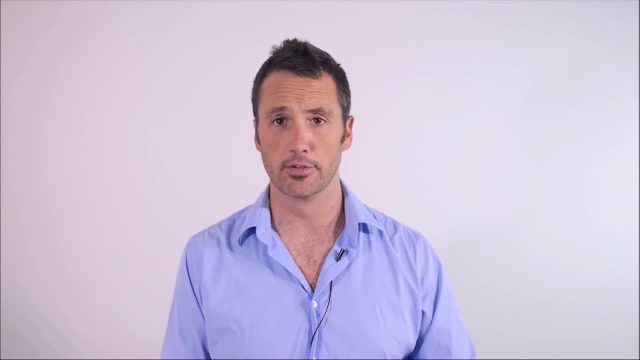 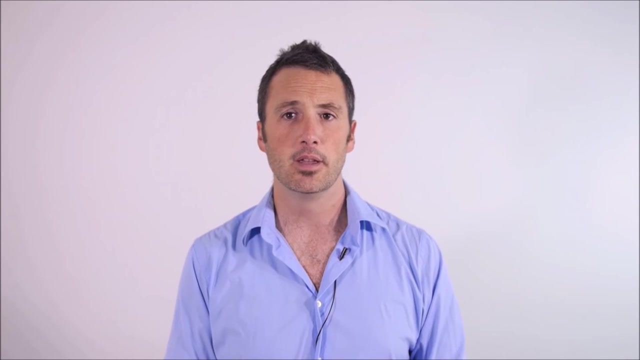 going to take two years to build a website, Nor should it cost $100,000.. Obviously, let's throw a scope of works in there. It's a simple website But really we can't judge unless we've predefined the measures, the metrics, And that's what a baseline is. It's basically. 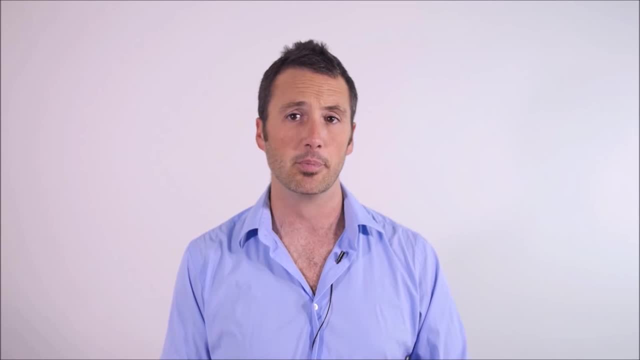 us estimating and getting approval for the scope of works. How busy is it going to be? What is it going to look like, What's the functionality, What's the attributes and so on? How long is it going to take? What's our schedule for this? How much money are we going? 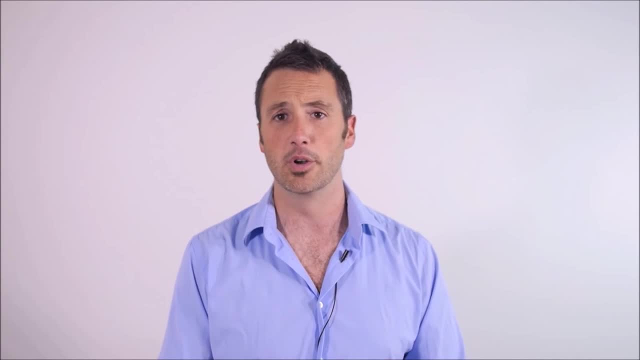 to throw at it. What's the budget? Quality factors and so on are common metrics used in baseline definition. By establishing these, by quantifying these, we can then measure, we can track the project, we can review it, we can identify how right we were And who. 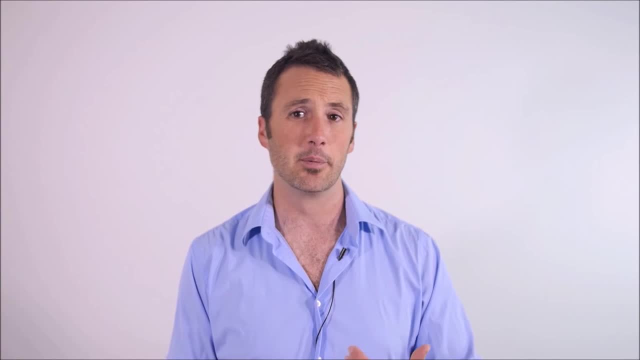 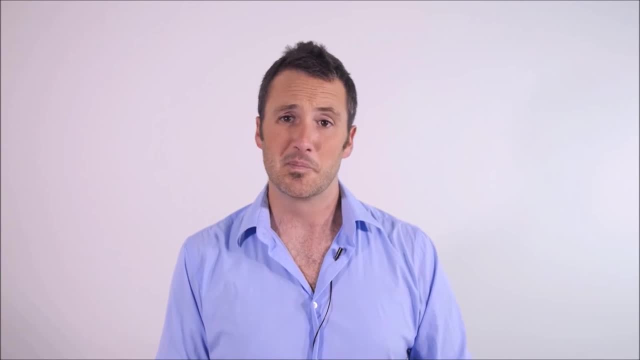 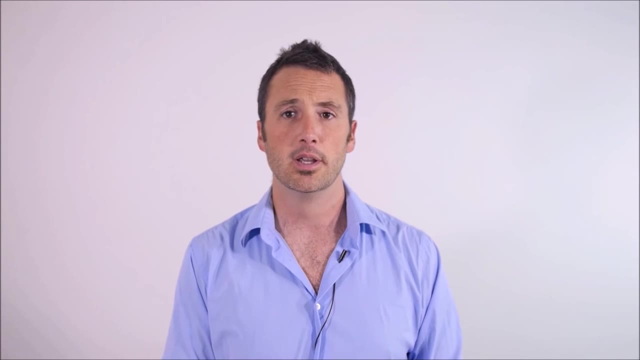 project well done. You go outside that Okay, there might be a few issues. It also enables the basis of comparative evaluation, So to measure project performance with without reports. we compare the plan with the actual And that allows us to understand how well we're going. 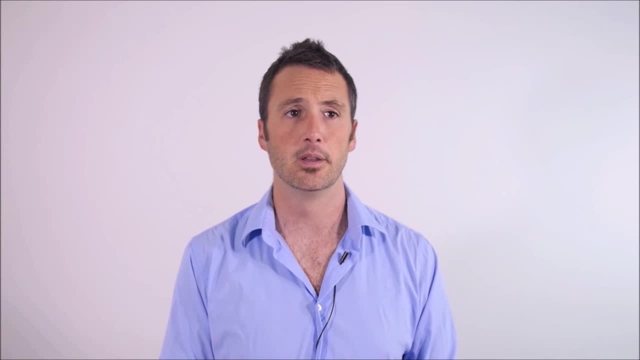 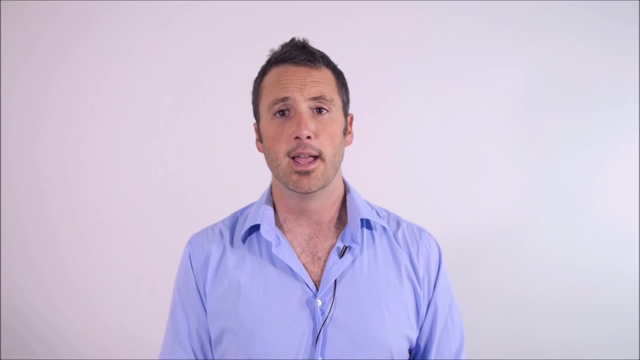 All this couldn't be achieved without initial baseline. So, in summary, a baseline is your plan, It's what you expect to do, It's what you've got, what you've got approval to do. Without it, it really makes project management and subsequently, 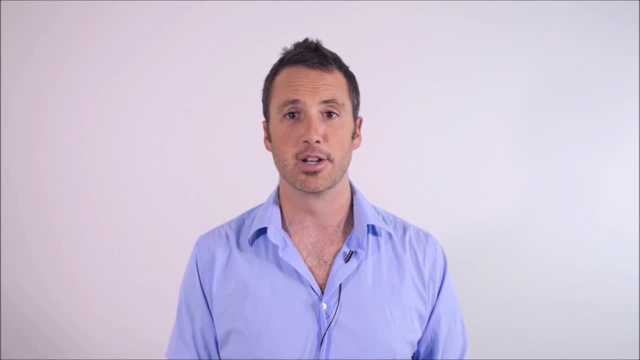 project evaluation a nightmare. It makes project handover impossible, especially when you haven't defined the scope. Cool, What I'll do also is I'll show you- because this is something I come across- a lot people fail an MS project to define a project baseline for their schedule. 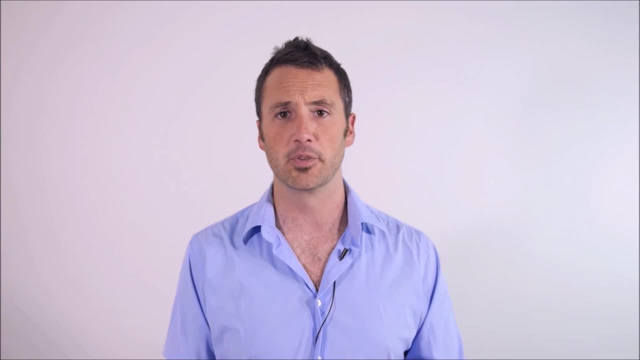 Then they start using the software and they work out that it's pretty much irrelevant. So stay tuned. In a link somewhere I'll put a video on how to make a baseline for MS project, And in doing so I've made myself committed to making more work. Great, Not well thought.